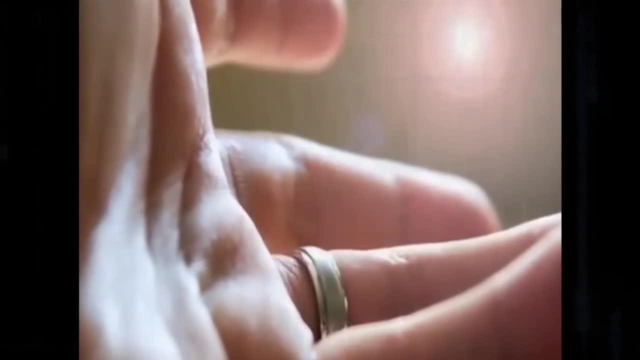 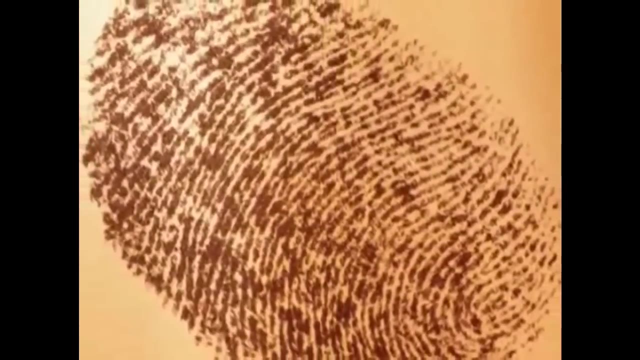 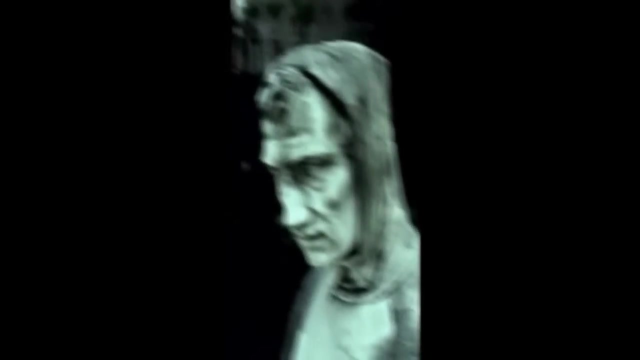 are the same. Everything we touch or make contact with is branded with a small expressed image, revealing to all who see it who was there. Around 1200 AD, a man named Leonardo Pisano, better known as Fibonacci, discovered a sequence of numbers that created a very interesting 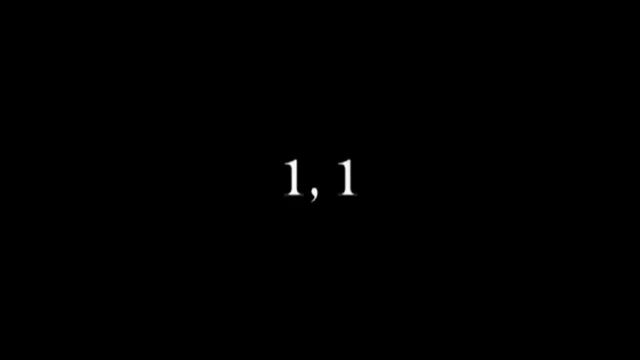 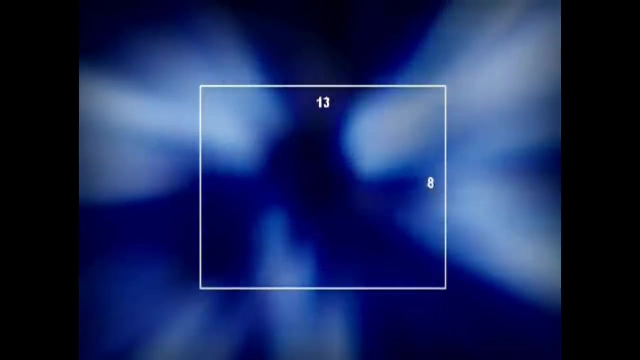 pattern. The sequence begins with the numbers 1,, 1,, 2,, 3,, 5,, 8,, 13,, 21,, 34, and continues indefinitely. Each number is obtained by adding the last two digits together, A rectangle with. 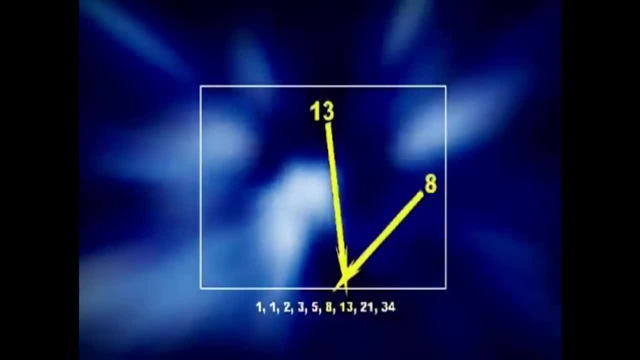 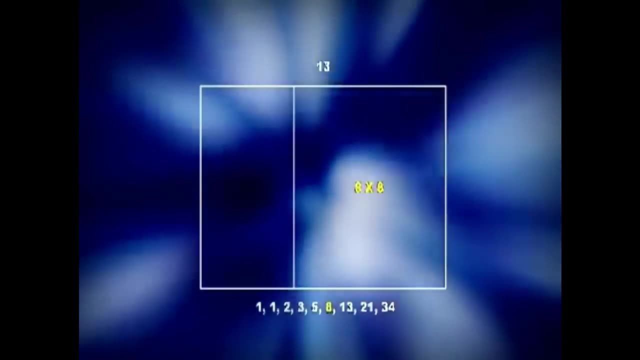 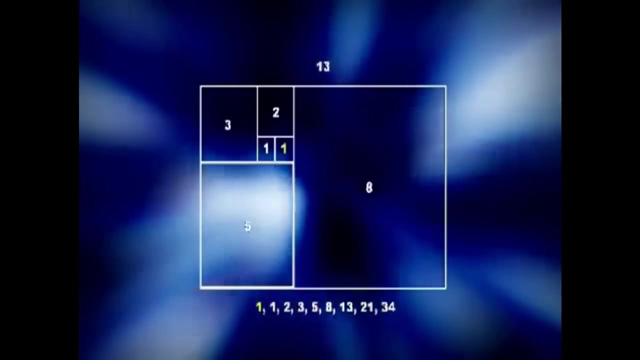 a length and width of any two of the numbers of this sequence forms what is known as the Golden Rectangle, a perfect rectangle, A Golden Rectangle can be broken down into squares the size of the next Fibonacci numbers, down and below. If we were to take a perfect or golden rectangle, break it. 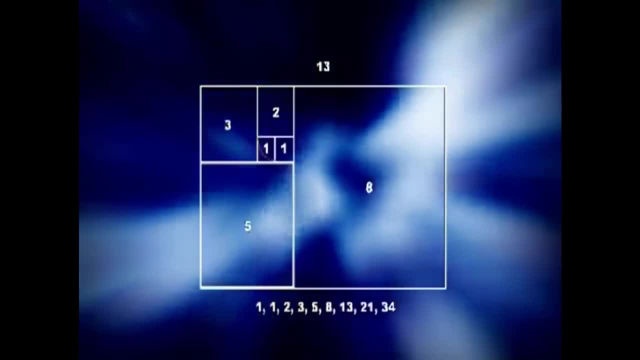 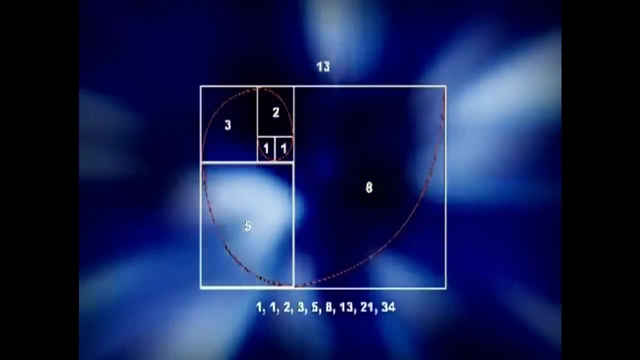 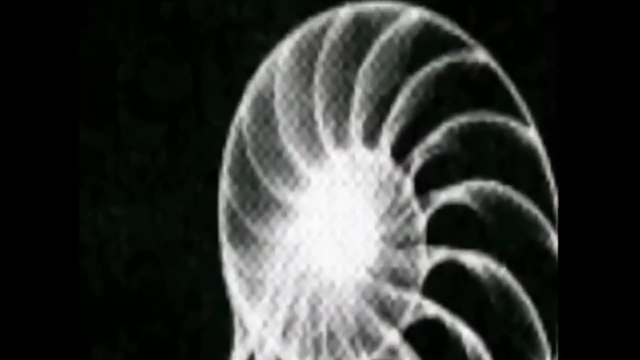 down into smaller squares, based on Fibonacci's sequence, and divide each with an arc. the patterns begin to take shape. We begin to see Fibonacci's spiral. The spiral in and of itself is insignificant. Its importance is revealed in where we find it. Take, for example, the sunflower, The display of its 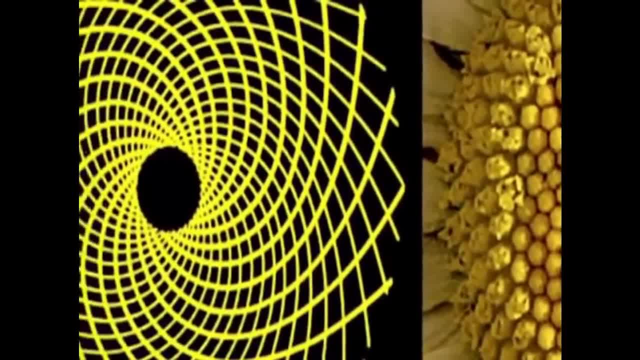 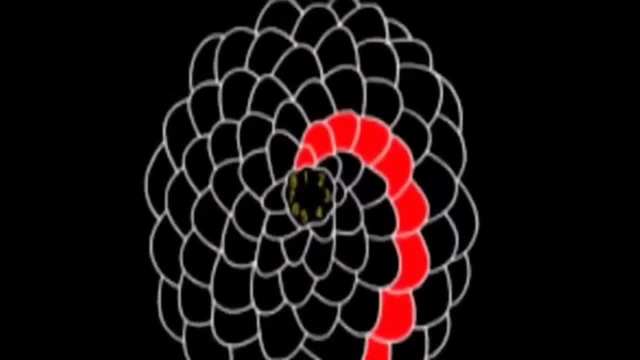 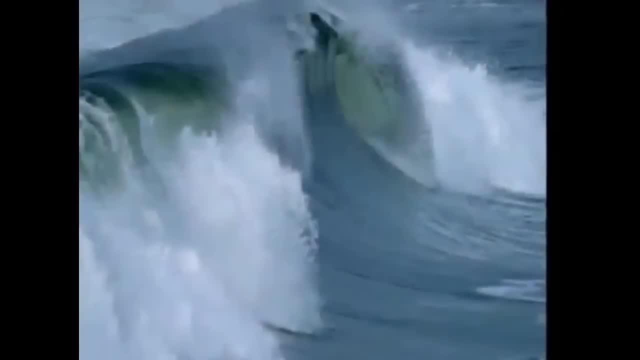 florets are in perfect spirals of 55,, 34, and 21,. the sequence of Fibonacci. The fruitlets of the pineapple create the same spiral. based on the sequence. The pinecone does the same. As currents move through the ocean and the tide rolls onto the shore, the waves that bring in the tide curve into. 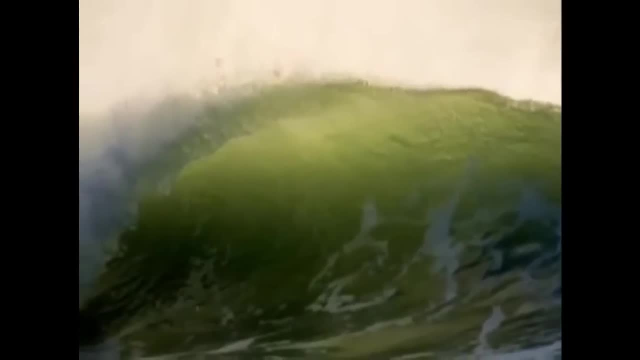 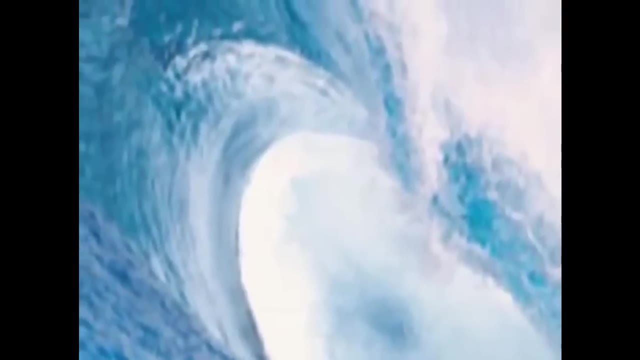 a spiral. that can be made into a spiral As the waves move through the ocean and the tide rolls into a spiral. the waves that bring in the tide curve into a spiral are mathematically diagrammed onto a plot at the points 1,, 1,, 2,, 3,, 5,, 8,, 13,, 21,, 34, and 55.. Buds on trees, sand dollars, starfish petals on flowers. 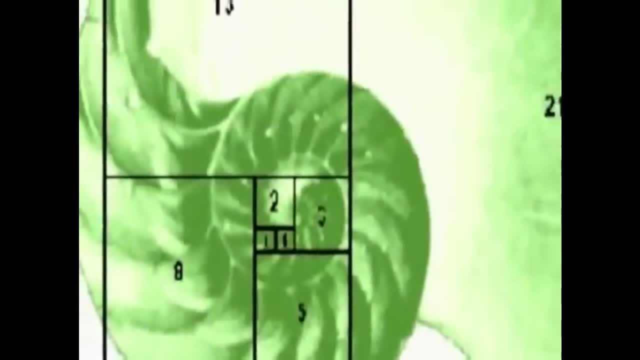 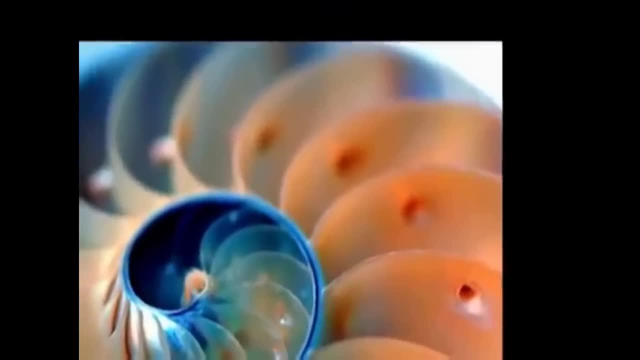 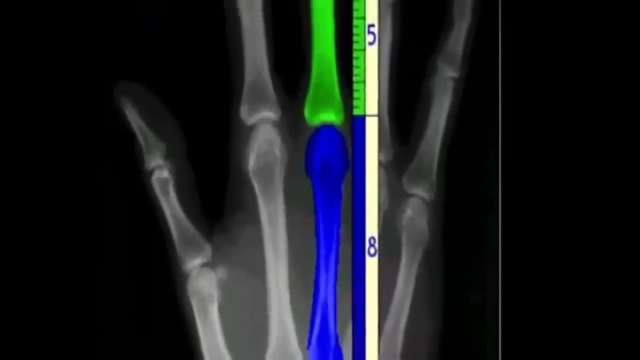 and especially the Nautilus shell, are formed with this exact same blueprint. With each segment of growth, the Nautilus adds to itself one more value on Fibonacci's scale. This blueprint can be seen around us on a small scale every day, but the greatest example of all is directly above our. 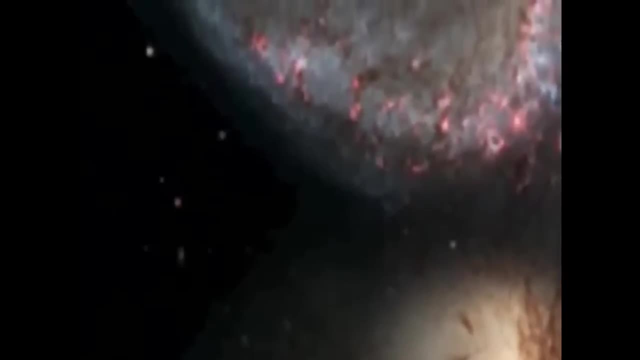 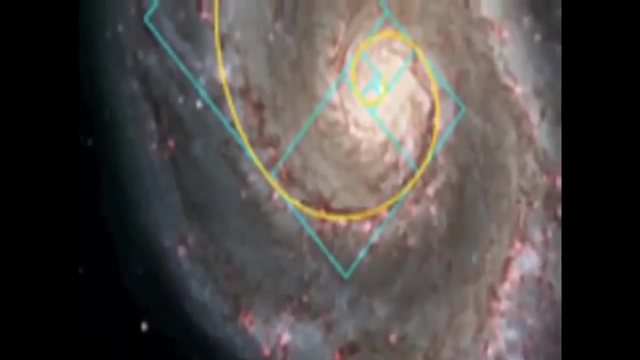 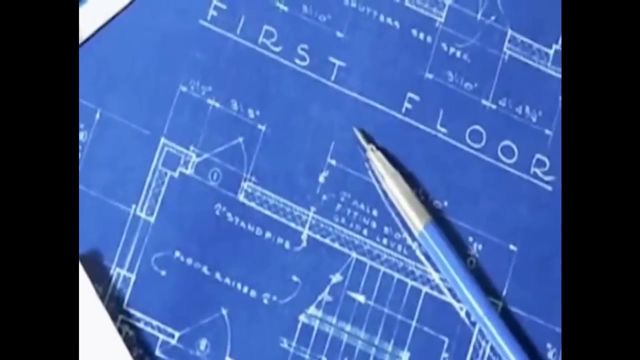 heads At an average of 100,000 light years across. even the spiral of the galaxies above us are formed with the exact design that the tiny shell is formed. This sequence, our blueprint, appears to be the trademark of a designer, a proof of a creator, Something left behind. 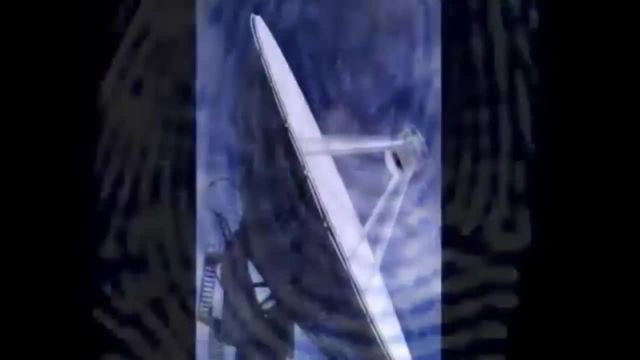 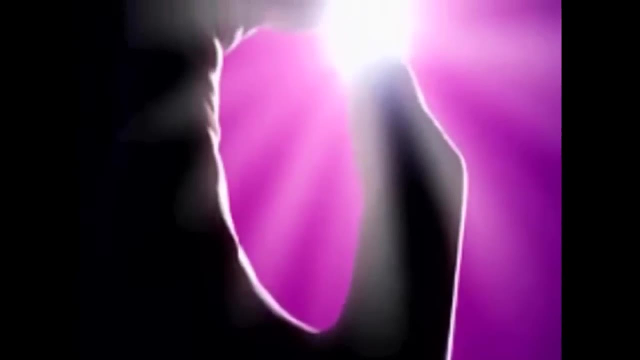 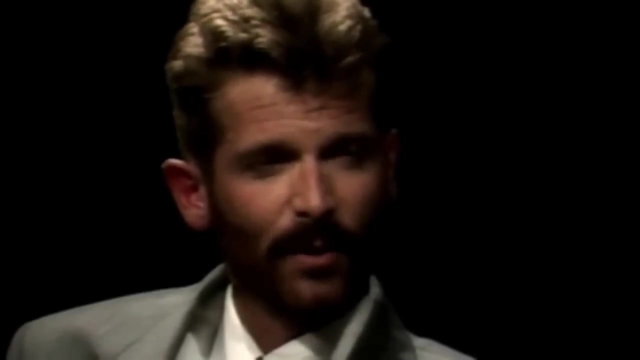 in the universe is a fingerprint. As we scan our universe, from the tiny flower to the awe-inspiring galaxy, we see the fingerprint of God. As you know, Mother Nature uses all kinds of mathematical languages. When we go to understand physical phenomena, we generally find that there's some. 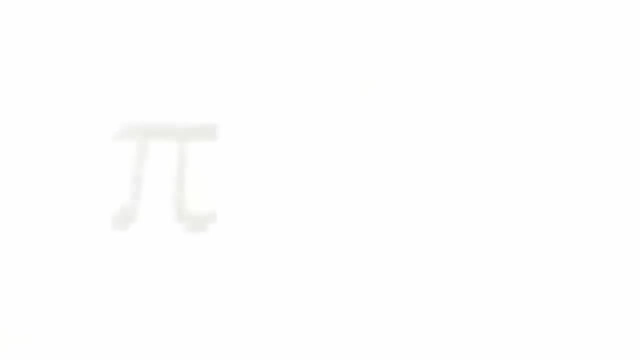 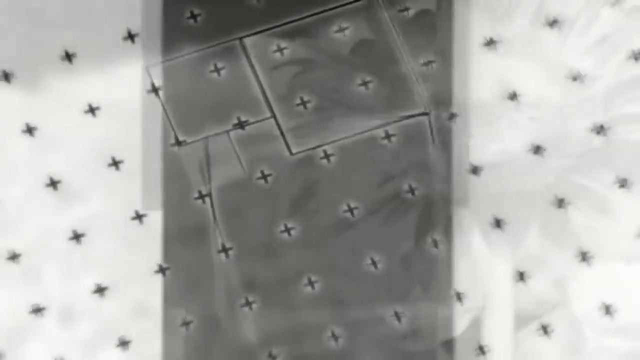 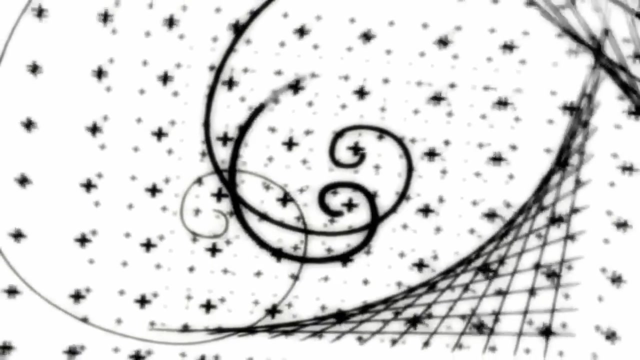 sort of mathematical underpinning to whatever the phenomenon is. You know, like the Fibonacci sequence, Just like that series you find in nature, Like the face of a sunflower. Where are the spirals? You see this math everywhere. How did we end up in a universe like that? 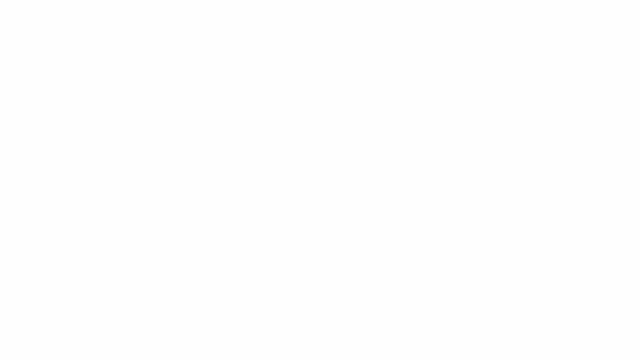 Why should the world behave according to, mathematically, yours? And it turns out, in fact, all of our senses appear to rely on sort of Fourier transforms, that they all seem to use the same mathematics. So again, here's evidence that the brain uses the same mathematics to decipher the sensory. 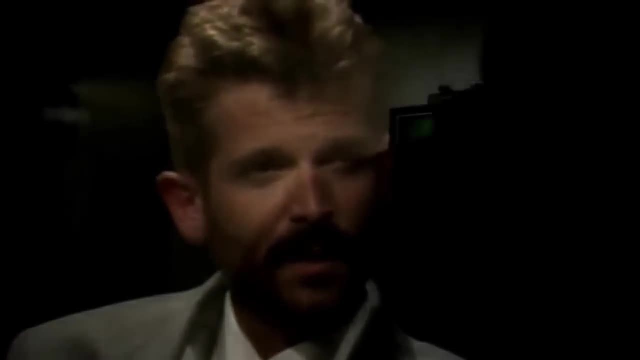 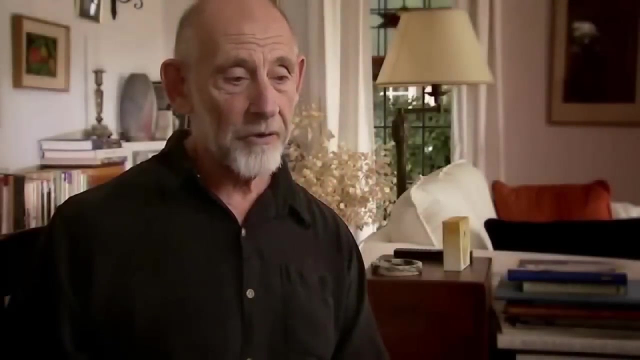 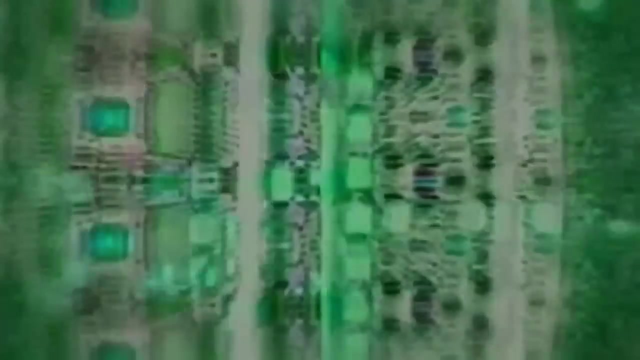 world, as they're involved in the making of a hologram, which is, as I say, not proof, but compelling evidence that something is going on there. Not only that, it becomes easier to describe with mathematics. as you go deeper and deeper into reality, mathematics becomes the only way to describe reality. 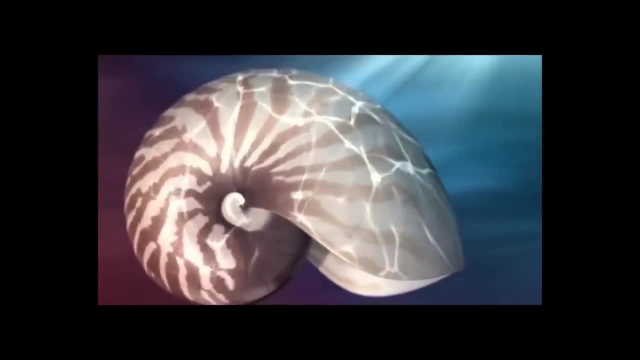 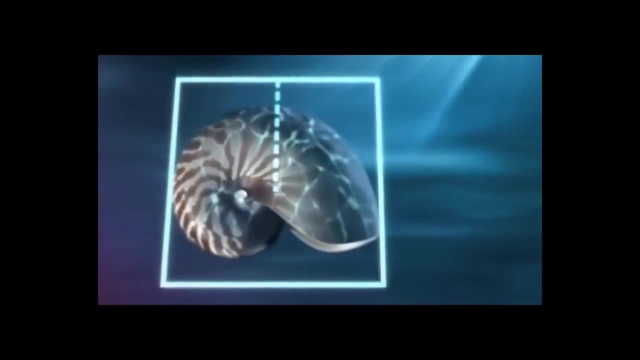 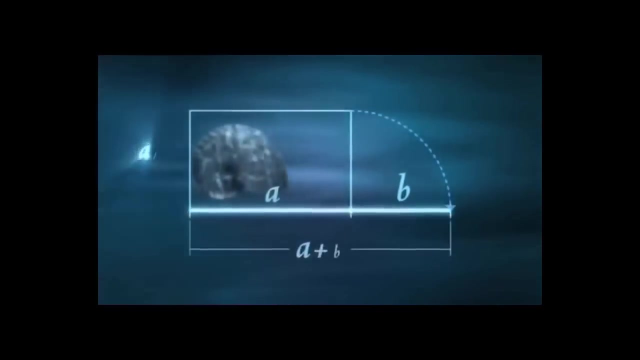 There's a conspiracy to hide this information. that DNA is a Fibonacci is an exemplification of this number or entity racial sequence, called the Golden Ratio, The ratio that proves the existence of intelligent design or the reality of intelligent design of the cosmos. I mean, if you go to the Golden Ratio site for Wikipedia too. on the same, 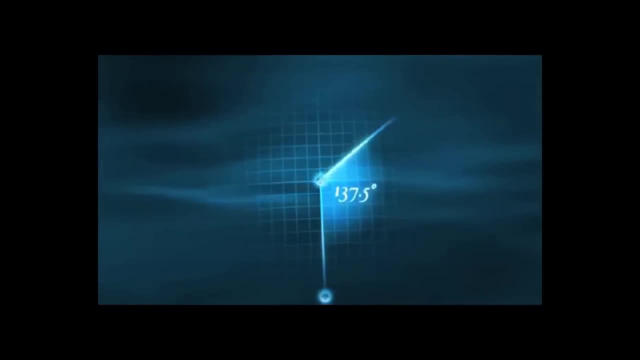 theme. they don't mention any of this stuff in nature that we're going to talk about here, that we talked about on the show two days ago and that we're talking about here. They talk about how it's found in architecture and math and all this kind of stuff. They. 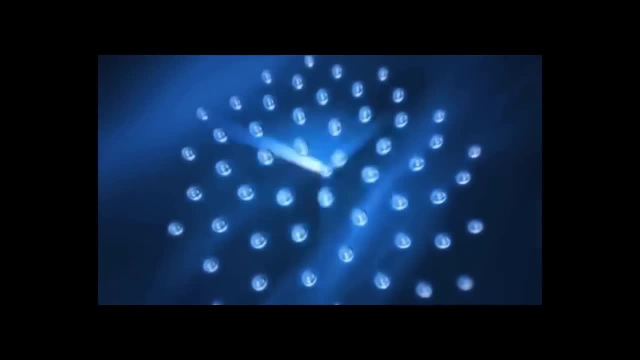 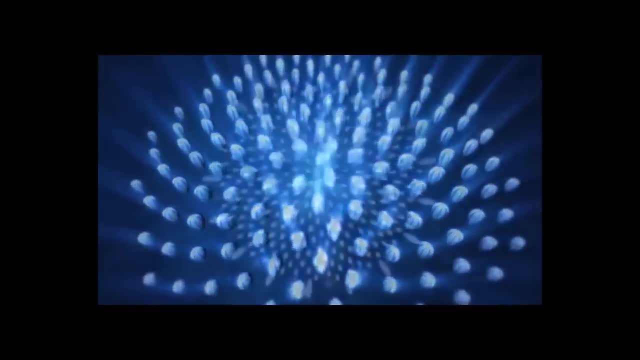 it's, it's, it's, it, it, it, it, it's, it, it's, it's, it's it's. I mean. well, that's the point here. I think that just made sense to me, thinking this through as I say it to. 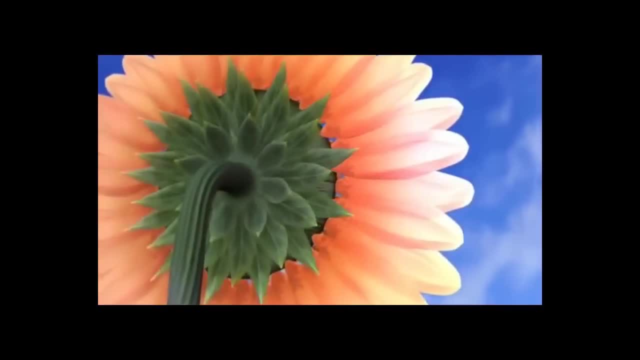 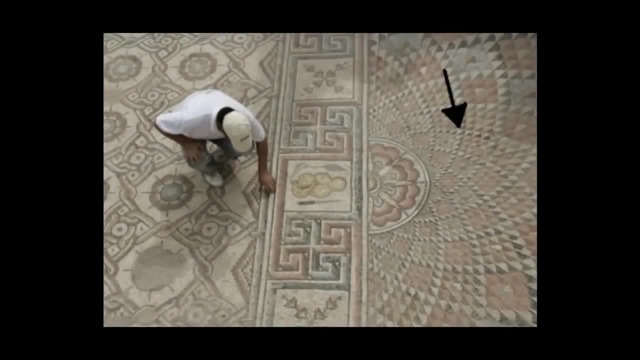 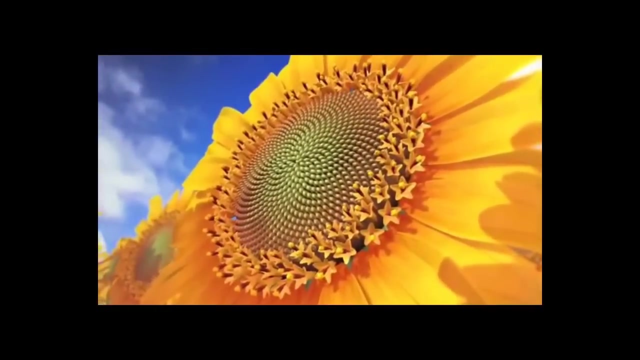 you. It has to be a conspiracy. How could all this be overlooked? and how could Wikipedia leave it out? It? it can't be. It has to be somehow. that big money has pushed their influence somehow and they've had a drive to keep this covered up or something. These 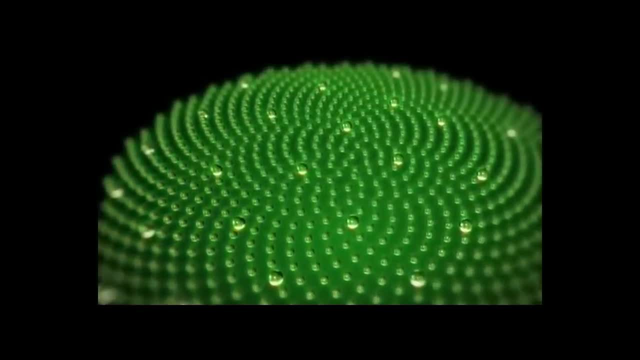 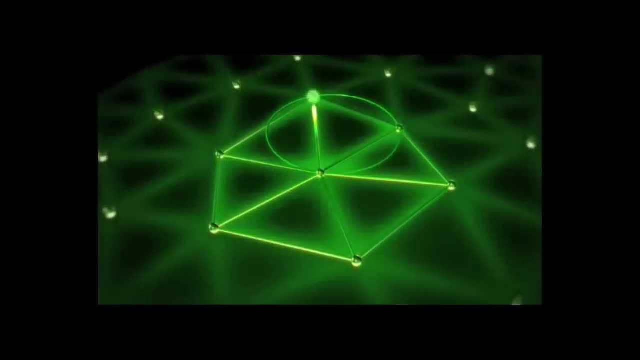 can't all be coincidences, and since they're doing that with everything else, it has to be the case that, uh, there's some movement to keep this stifled. i mean, why isn't- and here's another piece to add to this- why isn't this? in our education system, we learn all this junk geometry, p brain stuff. 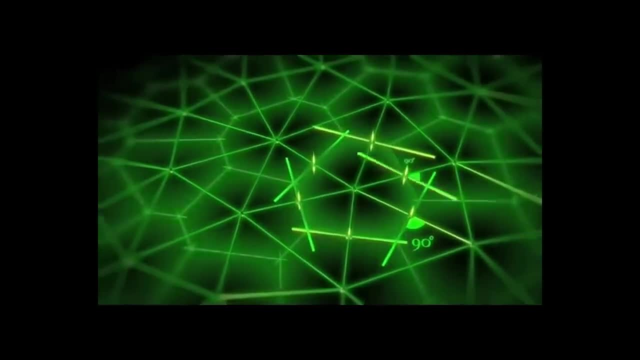 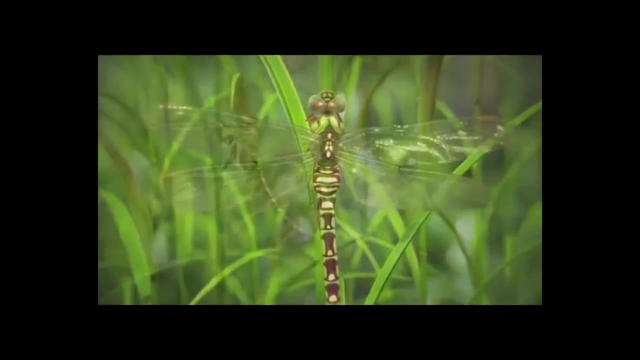 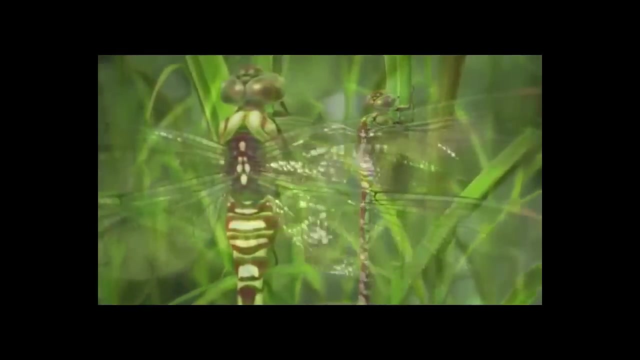 when you take geometry in high school and they don't teach you about any of this, the golden ratio everywhere in nature. i went through elementary school, you know. high school college- uh, you know. undergrad degree in college, uh, master's degree and halfway through phd, and never was. 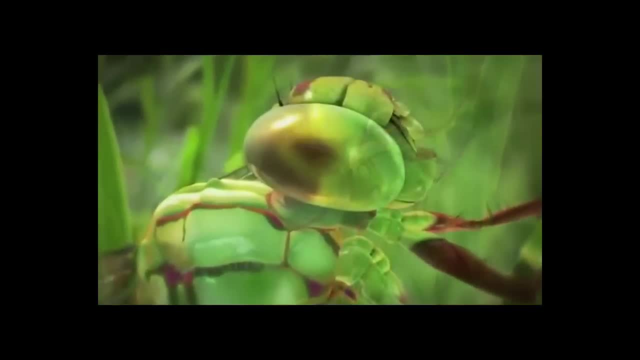 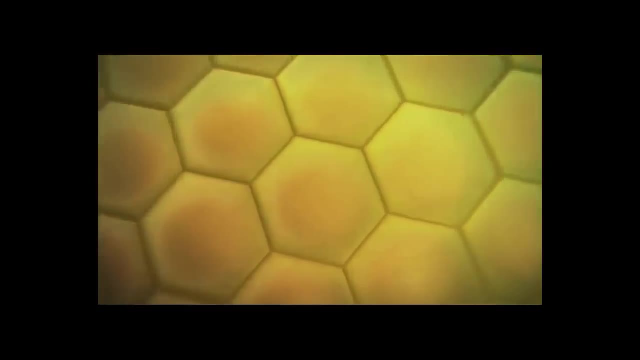 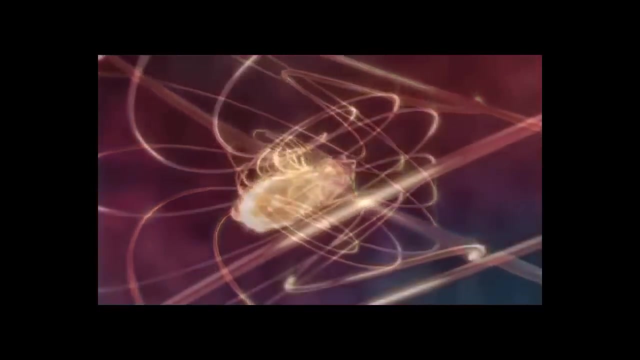 this, any of this mentioned. and we know who controls the universities: uh, the big money behind it, all the way up to the illuminati nephilim, uh, controllers. so this can't be. this is planned, okay, and you just wonder. it's gotta- i mean i'm almost concluding here- remind us davidson. 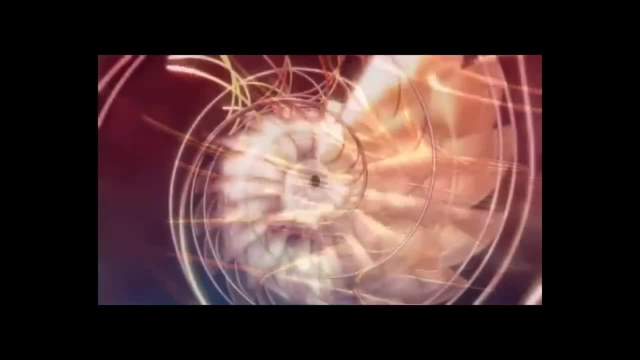 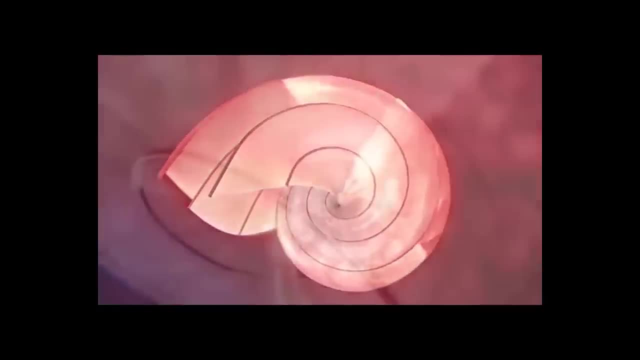 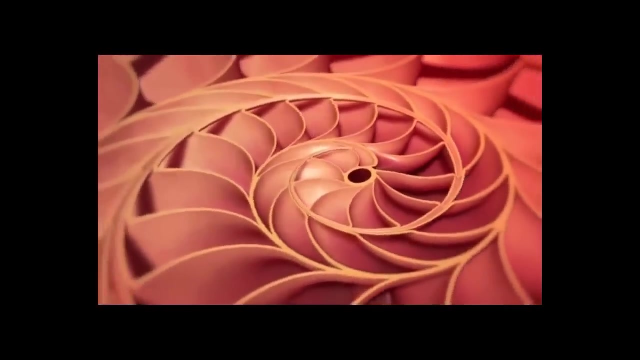 college site showing up number one in google all the time and first page, and wikipedia having the strange measurements which don't correlate with all kinds of these examples from academics that i'm finding. i'm putting them all pictures of the screenshots and the newsletter. it's got to be a conspiracy. i mean we could keep going compiling the evidence, it would just all. 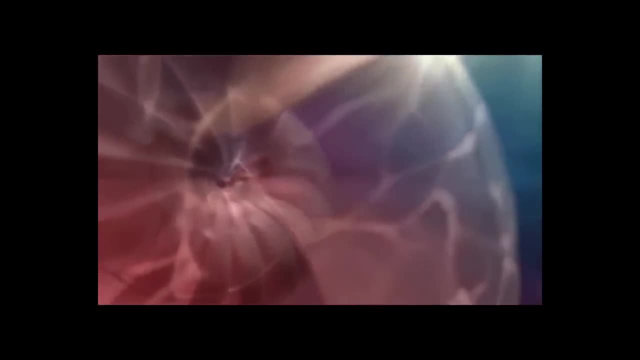 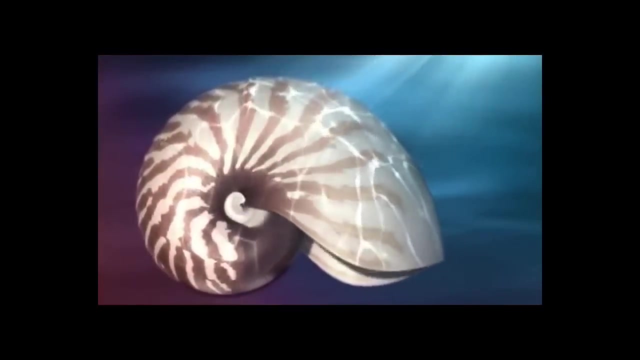 lead to it so and that, and if we could keep compiling evidence of it being a conspiracy. i mean, everything points towards it. I'm just throwing ideas off the top of my head. These strange sites show up on top. Wikipedia is wrong. it's covered up completely in the best-selling. 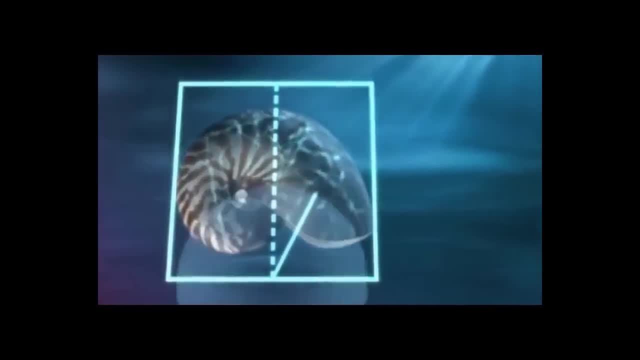 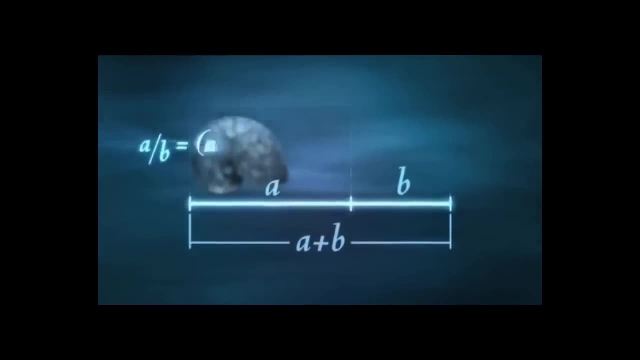 books about the Golden Ratio which come from wealthy university professors. It's the university's and education's government-controlled education system absolutely covers it up. You see how many everything's falling in the same direction. So when everything all these conclusions point to the same direction, that it's covered up and hidden. 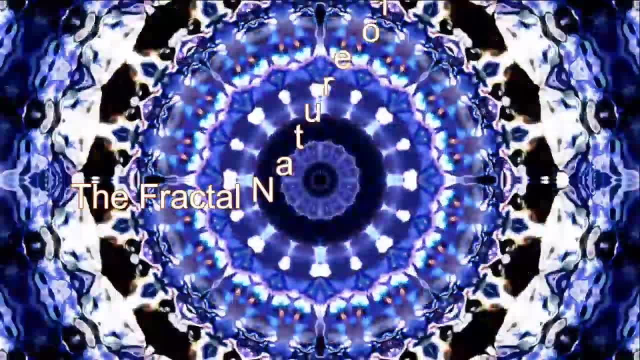 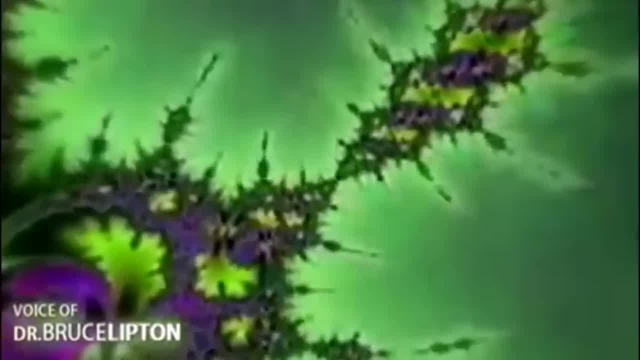 The geometry. the structure of nature is designed on the basis of what is called fractal geometry, And fractal geometry is unique geometry, not the one we learn in school. The geometry we did learn in school called Euclidean geometry. you can't model nature with it. All those 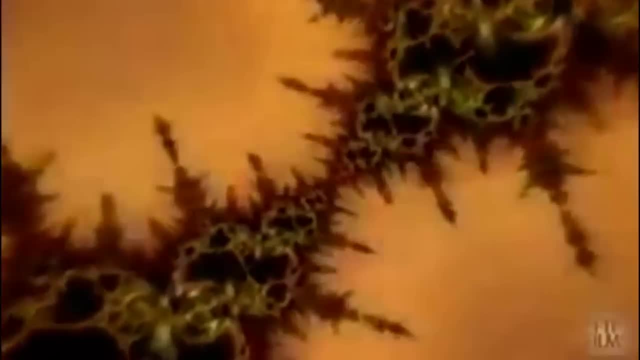 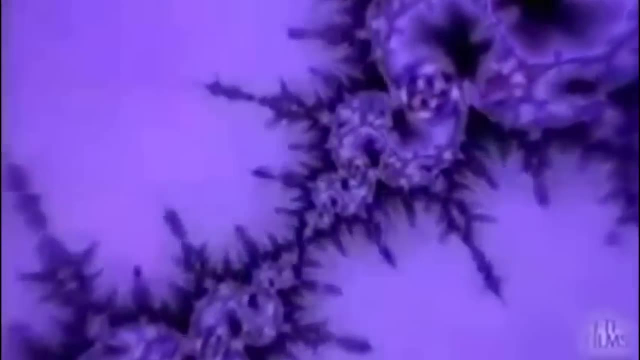 triangles, cones, cubes and spheres are not what nature really looks like. but when we were five years old In kindergarten, we made a tree, we made a tree, and we made a tree and we made a Euclidean tree. We had like a cylinder for the trunk and a ball for the 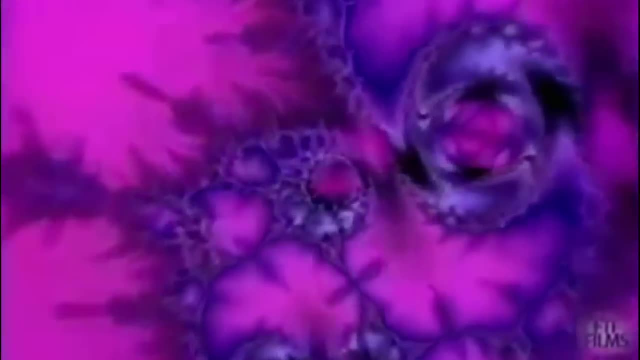 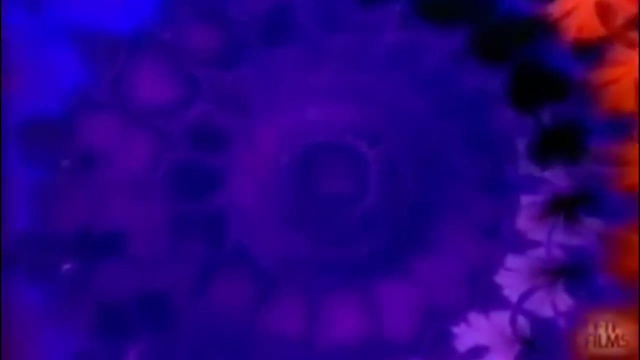 top, But obviously that's not nature-like. That geometry is not the nature geometry. We now recognize this new geometry that really came into our world in 1983 with the work of Manuel Mandelbrot from IBM, called fractal geometry And it's a different version of 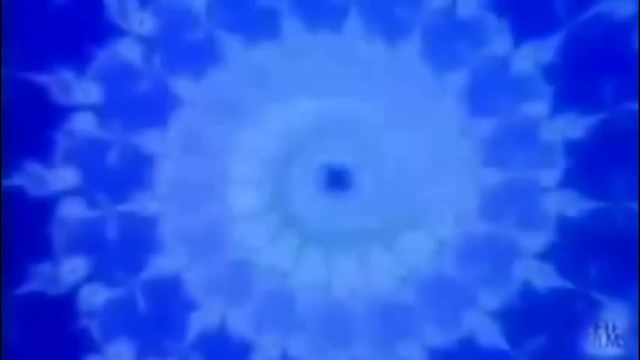 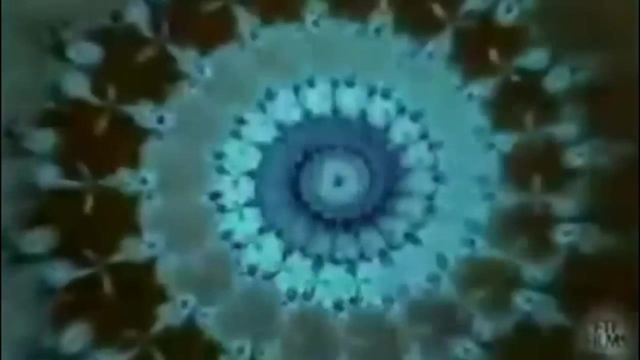 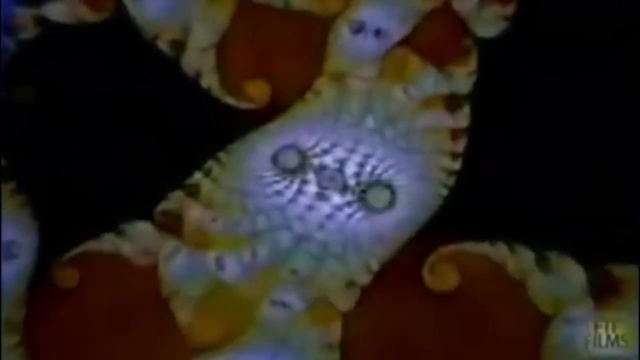 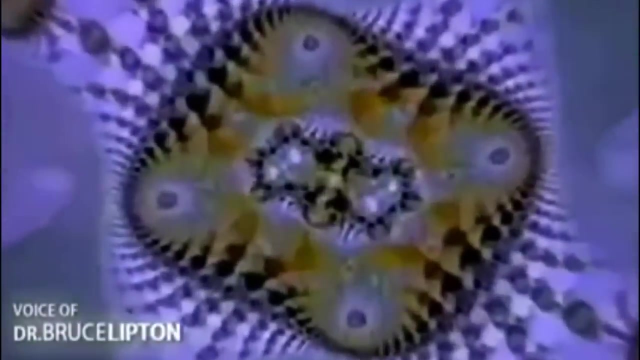 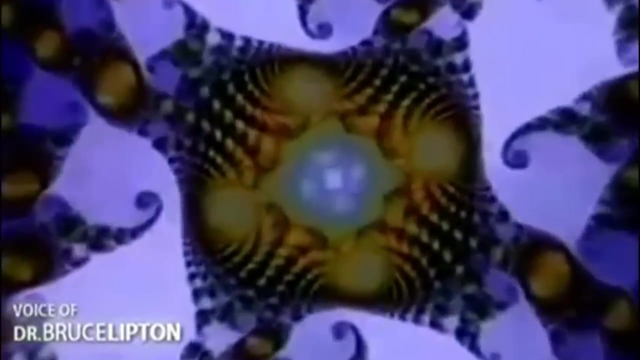 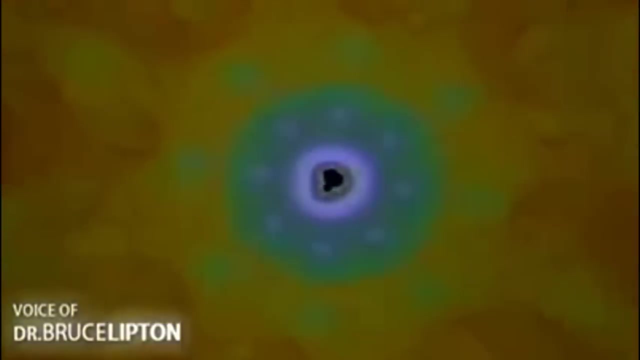 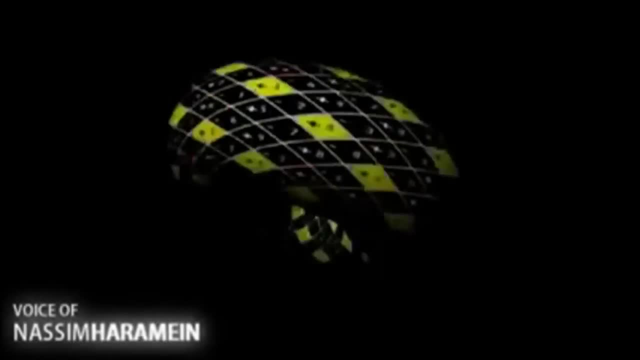 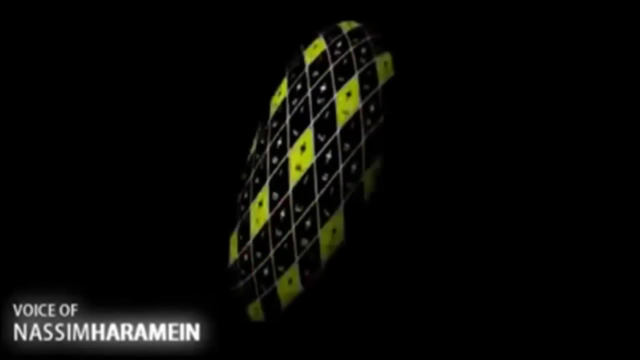 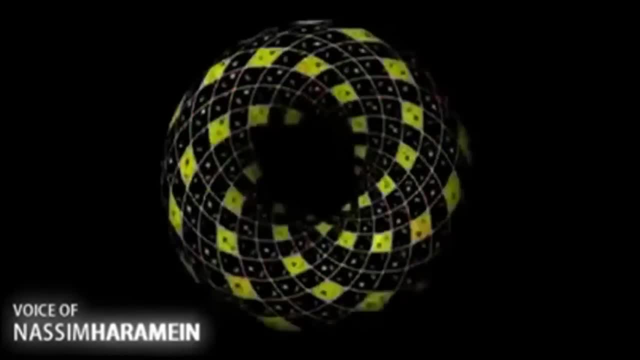 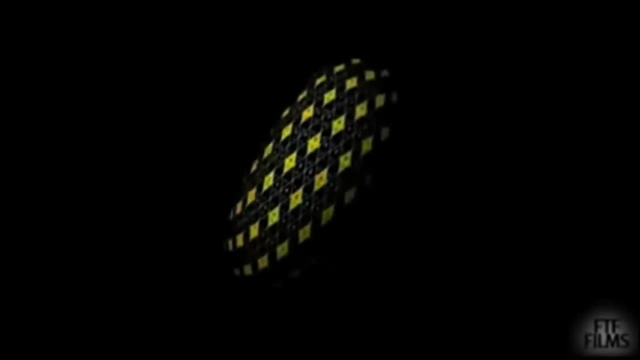 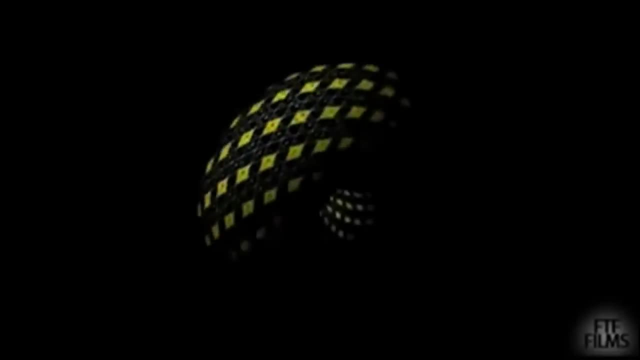 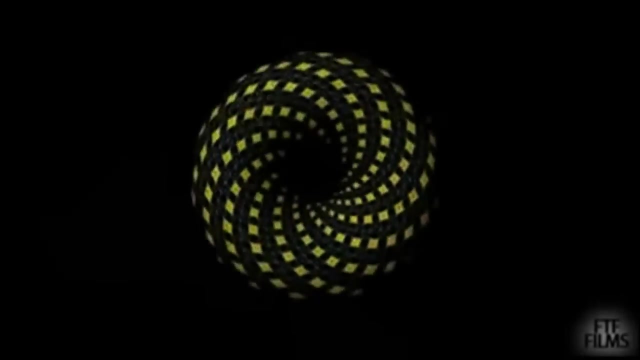 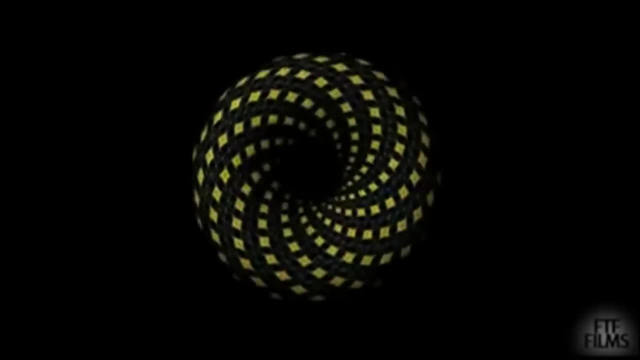 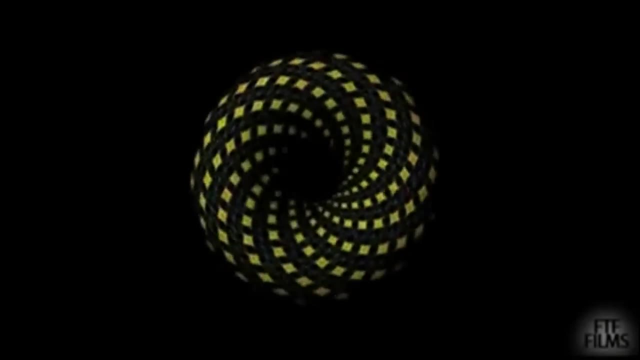 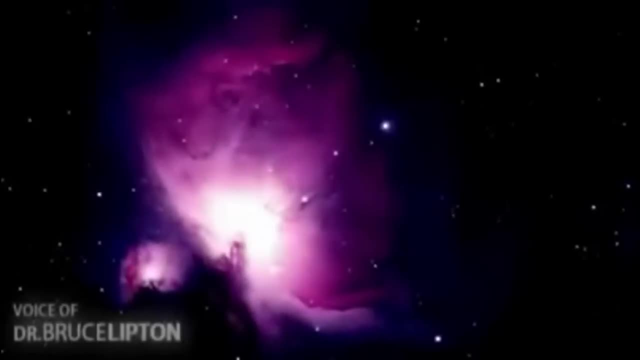 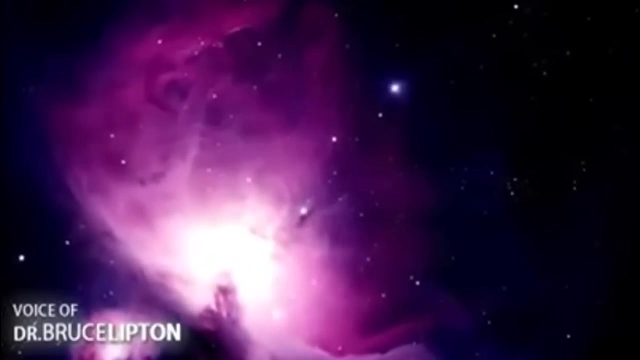 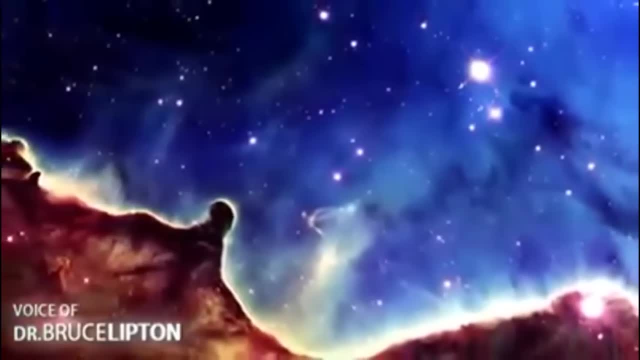 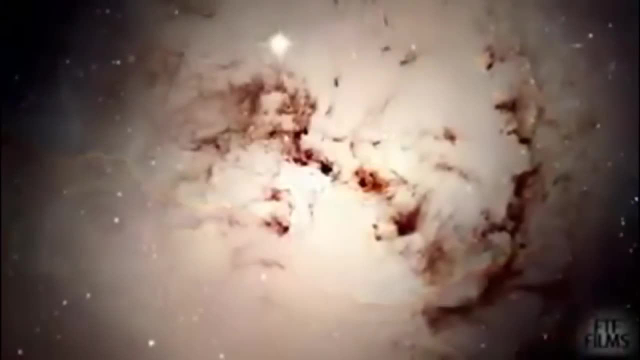 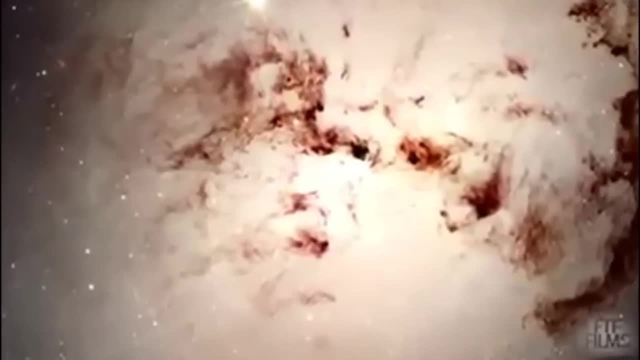 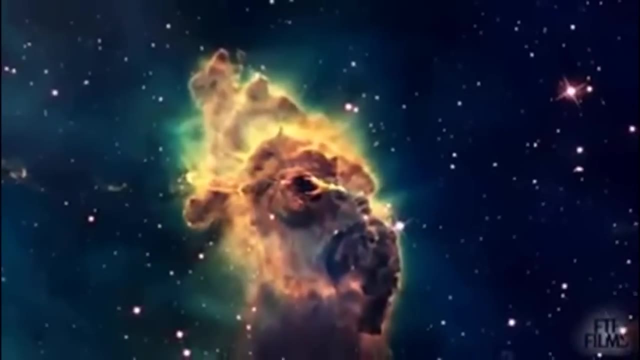 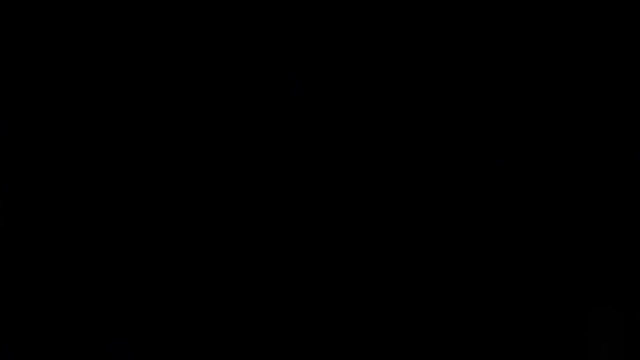 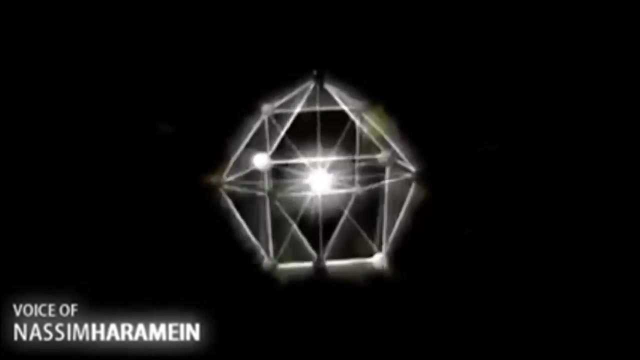 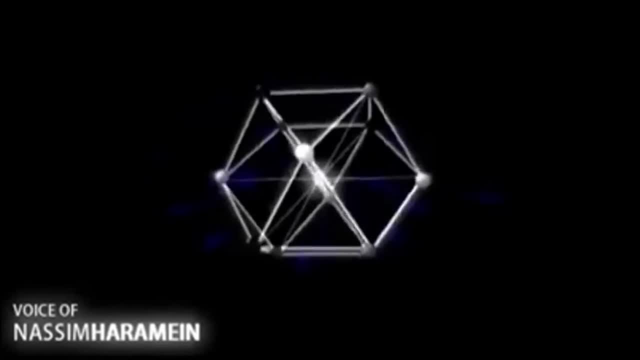 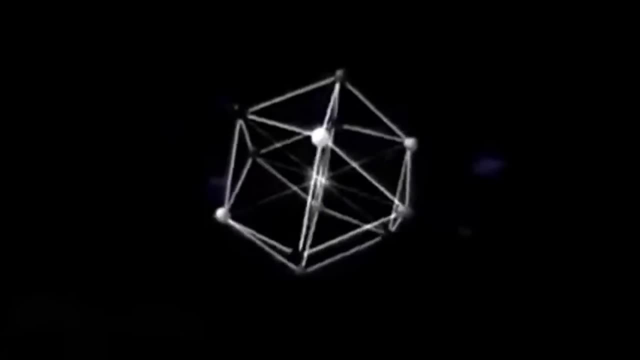 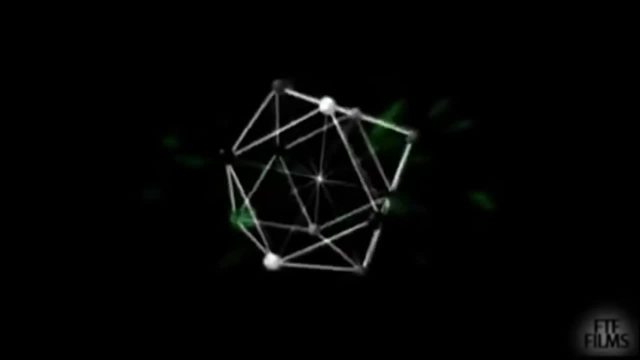 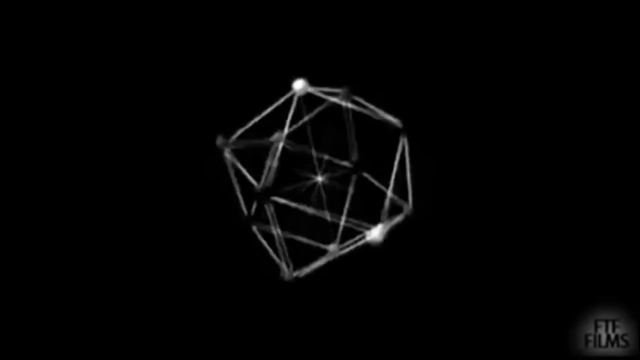 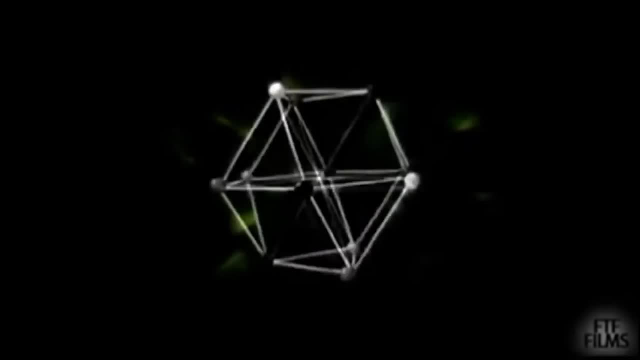 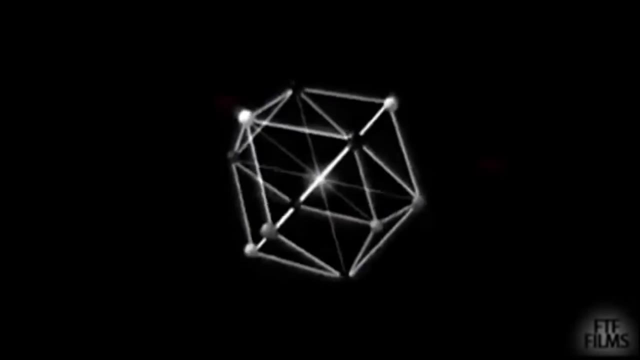 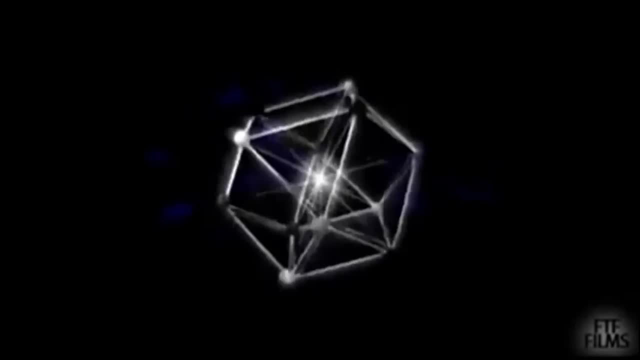 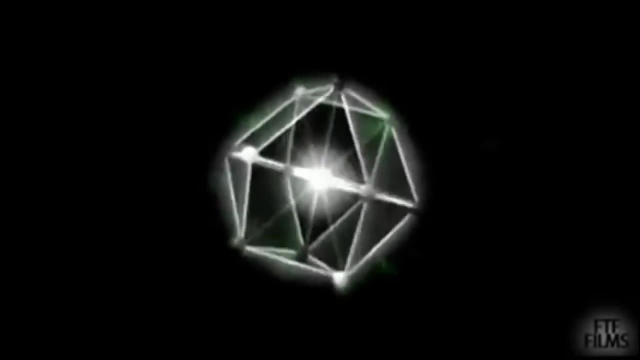 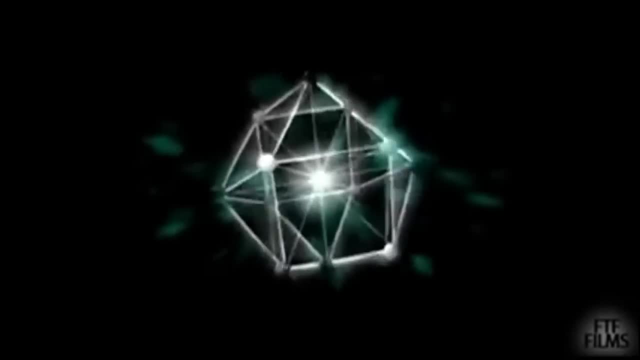 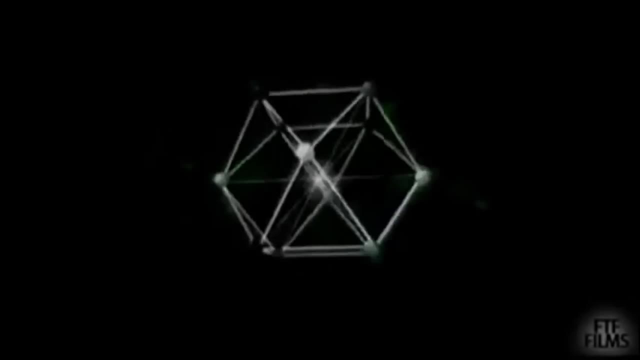 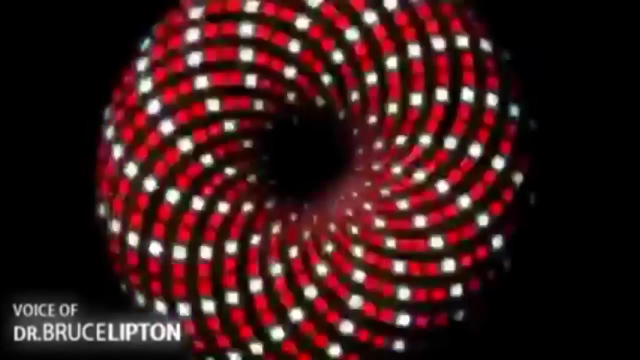 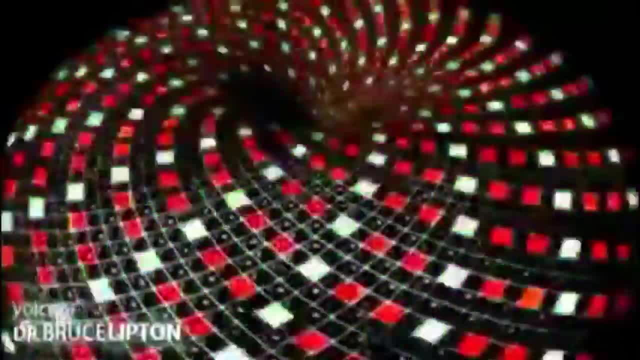 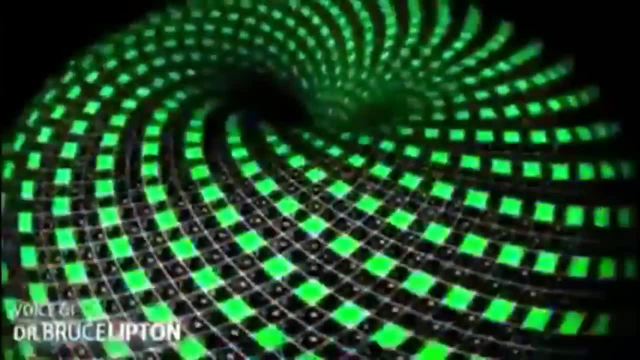 that we have in our own world, in the world where we live, so that it becomes understandable. This is why, for example, why we work on cells in biology: because if we get an understanding of the nature of the cells, we can apply that information directly to the nature of human. 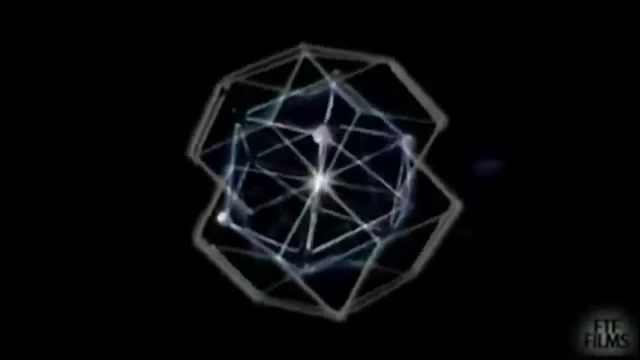 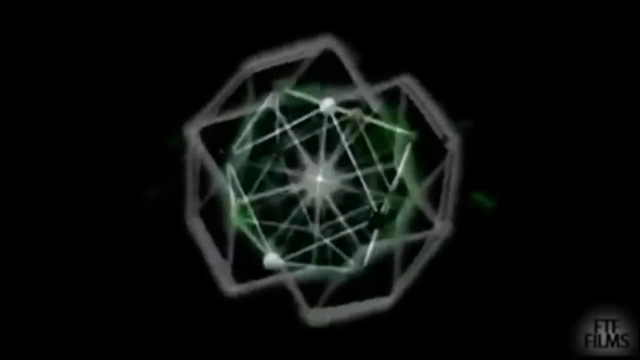 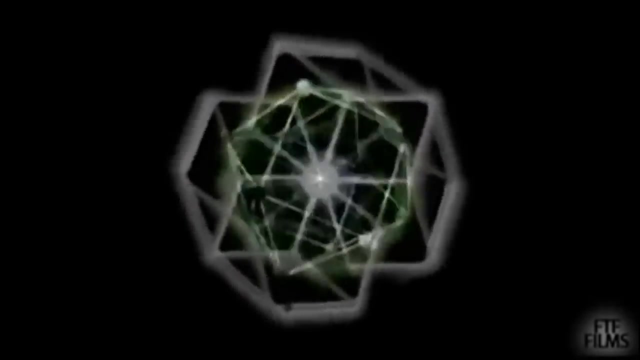 biology so that we extend this work. So in looking at nature's fractal and recognizing that the cell is the fundamental unit of the human body, that the human body is actually built in the image of that cell, then we start to recognize inside of you right now are 50 trillion citizens. 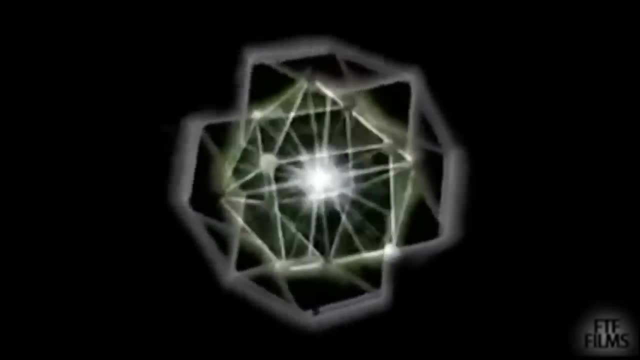 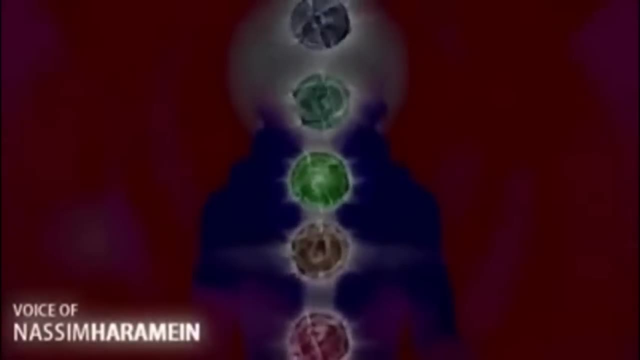 Each cell is its own sentient being. When I was culturing these cells, I'd take them out of a person's body, put them in a culture dish and they have their own life. They didn't need us. It helps. It helps to get other physicists to look at it, to get some credibility in the physics. 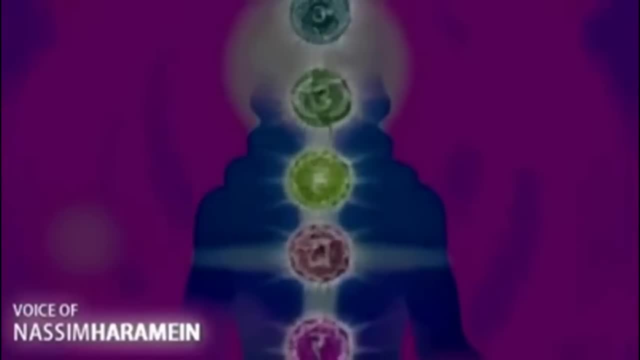 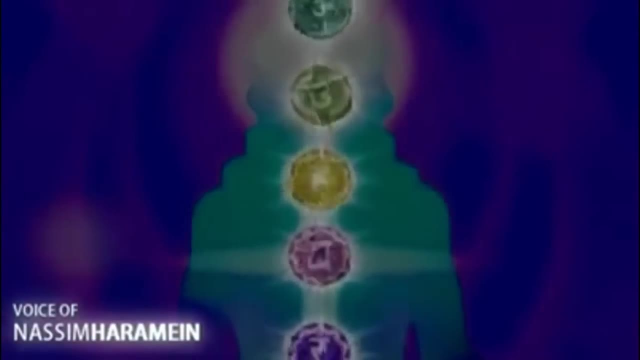 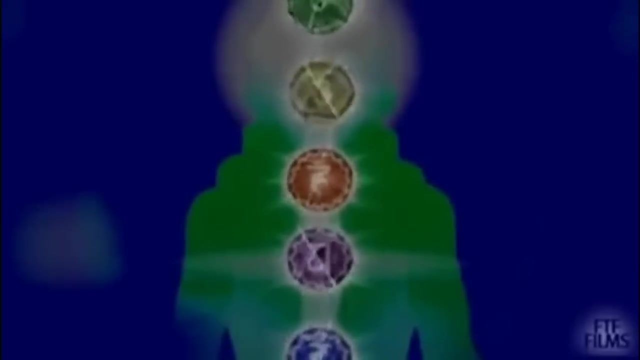 I'm writing and to make people aware that we are not living in a finite world, that the atomic structure itself has this infinite potential within it, that when people are talking philosophically or spiritually about their infinite nature and all this stuff, it doesn't have to be outside the physical world.